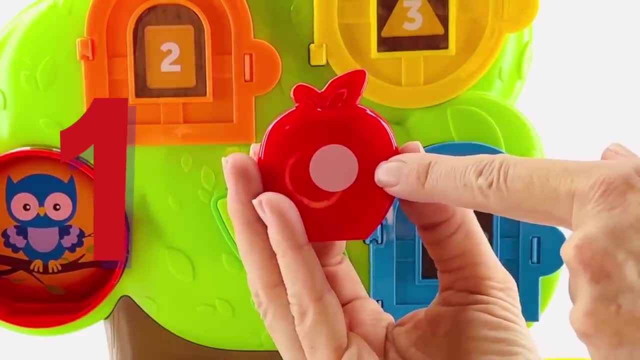 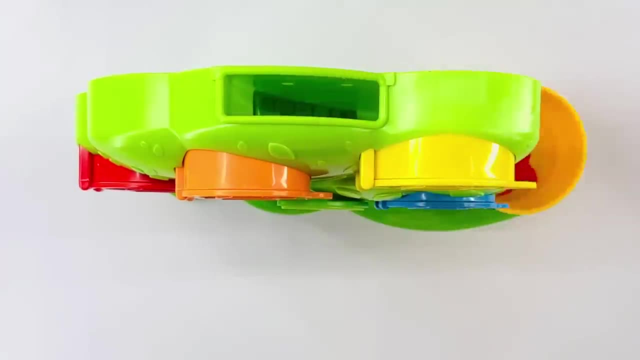 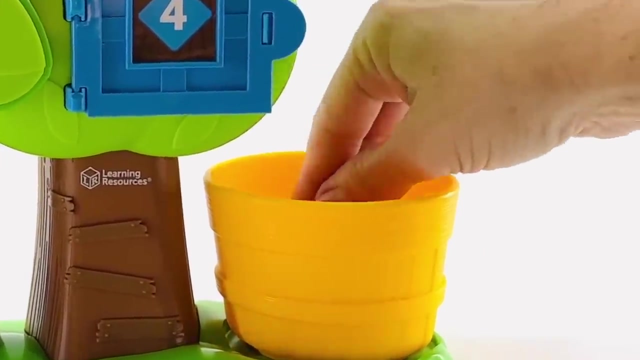 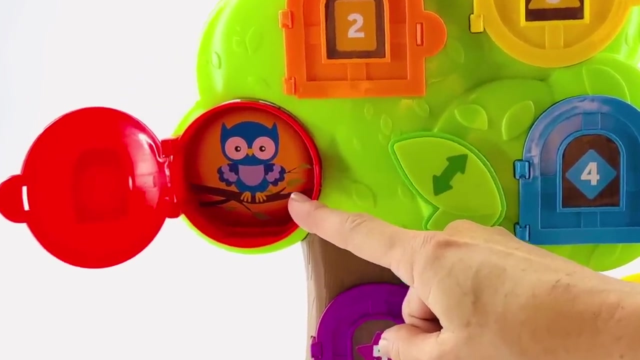 This apple has one dot. Great job. Now let's put it up here in the top of the tree and see what happens. Hey, It fell here in the bucket. Let's keep it right there for now. What's that inside of the door? That's an owl. Do you know what an owl says? An owl says: 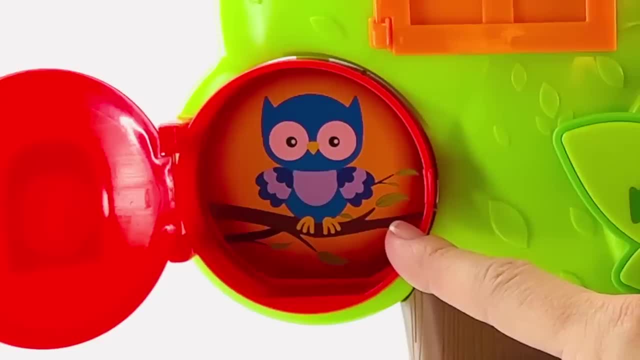 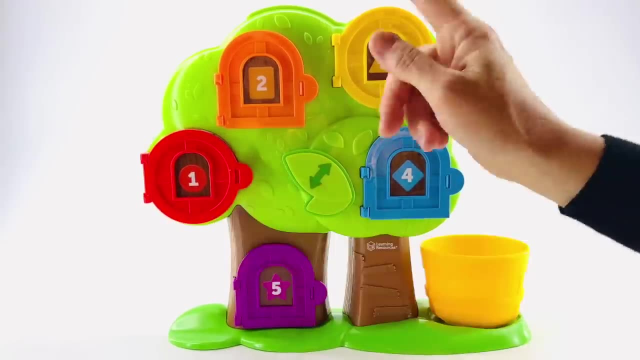 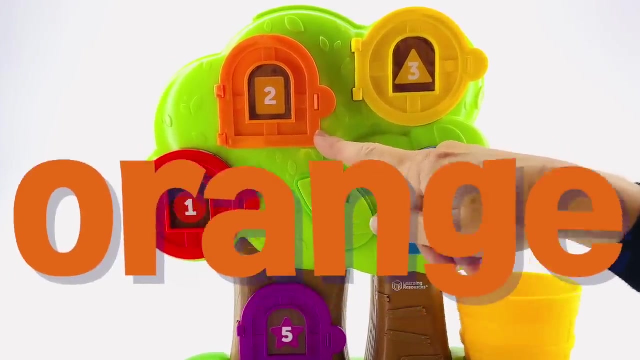 hoo hoo. An owl is nocturnal, which means it's up during the night and sleeps during the day. Let's let it go to sleep. And now let's look at door number two. That's the number two. Do you know what color this is? That's orange. Orange. in Spanish is anaranjado. 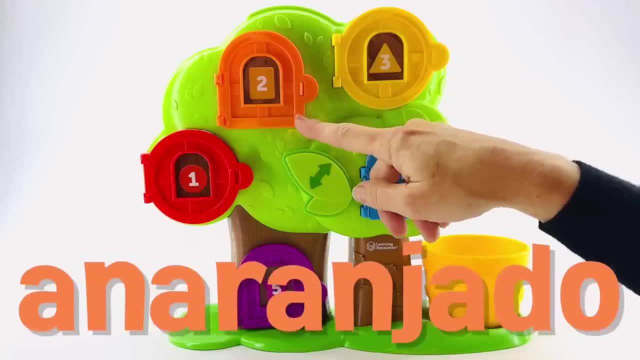 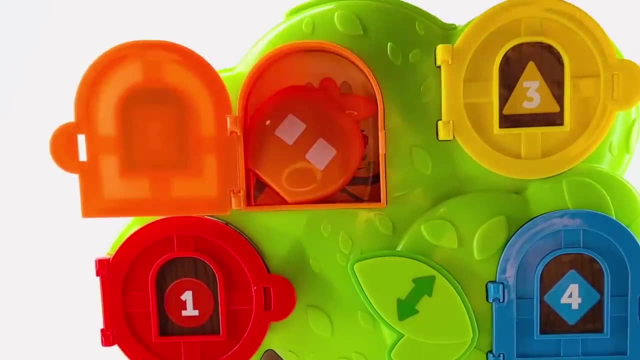 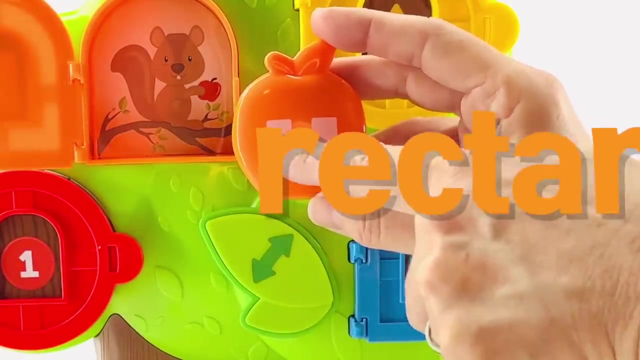 That's a really long word. Let's say it again: Anaranjado. Okay, let's see what's inside. Hey, It's another apple. Let's see what's on this one. This one has two rectangles. Let's count them together: One. 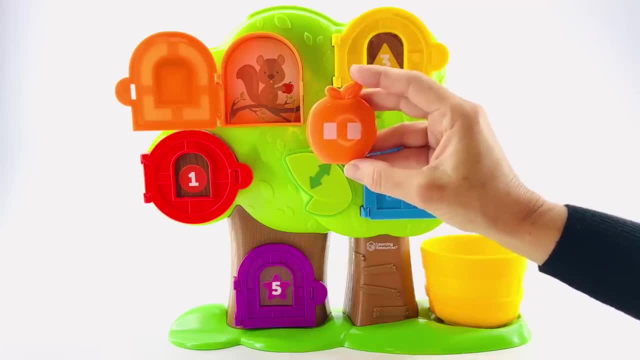 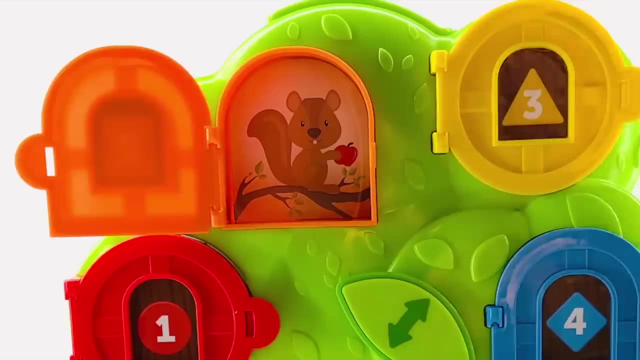 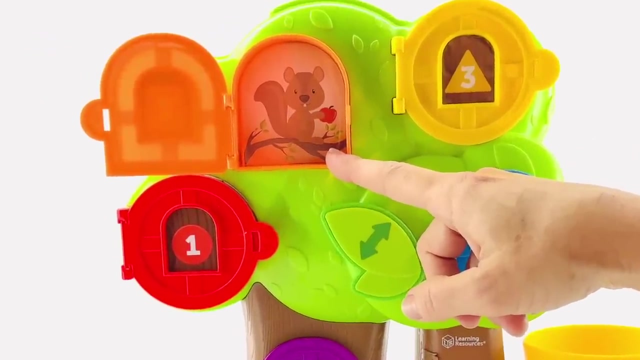 two. Great job. Let's put it back in the tree and see if it falls in the basket. Yes, There it landed. What animal is this? That's a squirrel. A squirrel loves to live in a tree and it loves to eat nuts and lots of other treats. 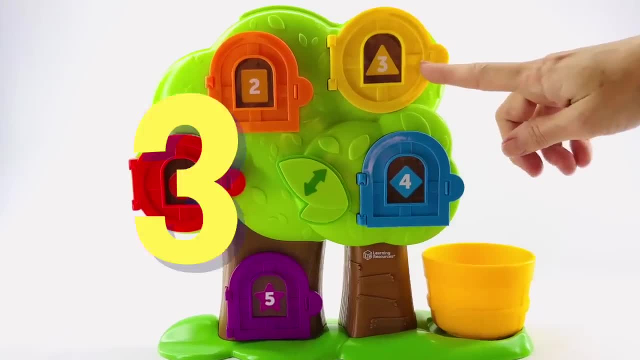 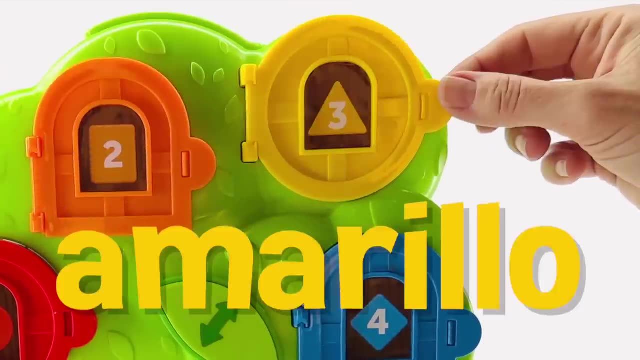 Okay, let's see what's next. That would be number three. Do you know what color this is? Do you know what color this is? Do you know what color this is? This is yellow. Yellow. in Spanish is amarillo. Let's say that together: Amarillo. 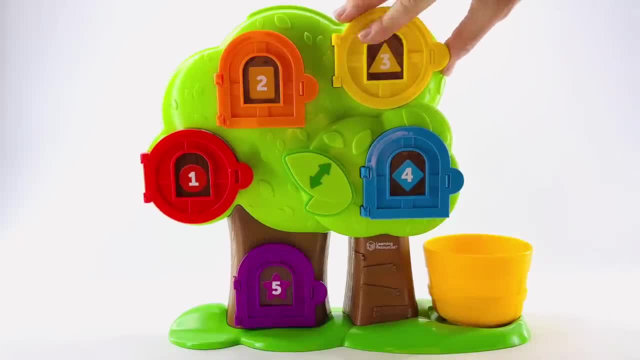 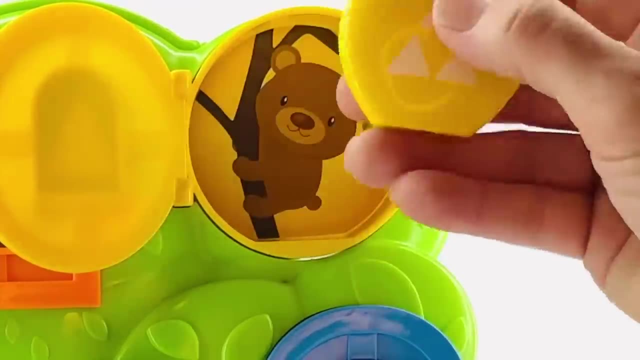 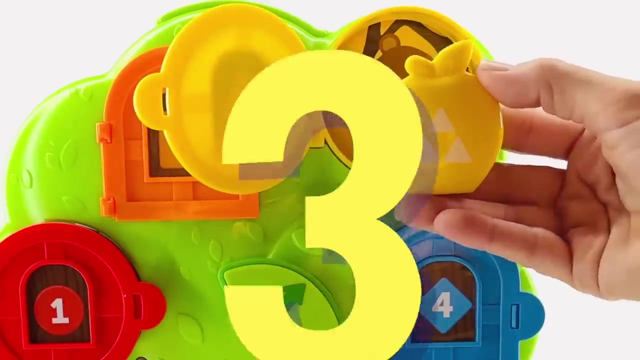 Okay, let's open it up and see what's inside. Hey, It's another apple. This apple has three triangles. Let's count them together: One, two, three, Three triangles. Okay, are you ready to put it inside the tree? 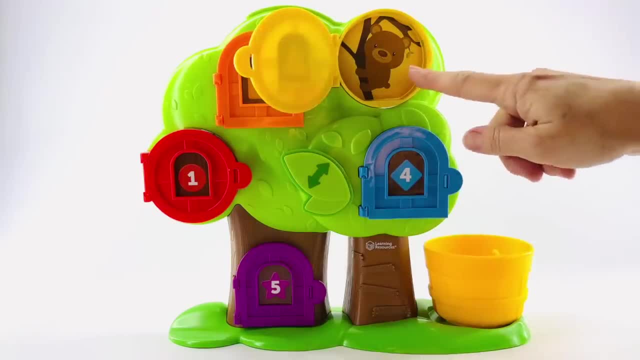 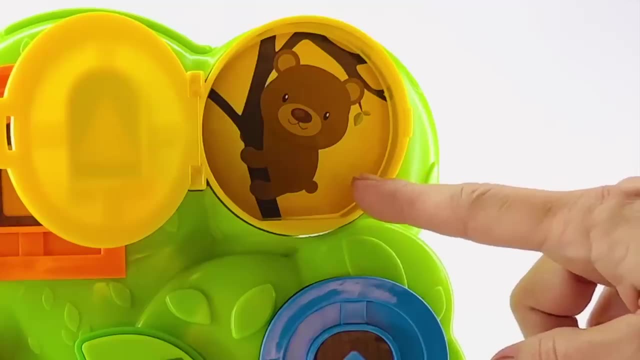 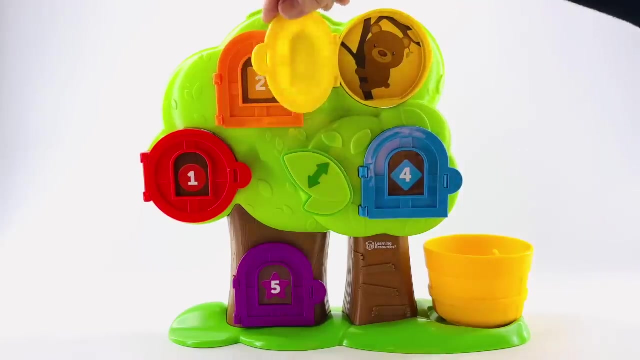 Great. It landed in the basket And here's a bear. A bear is in the tree. A bear roars really loud. Can I hear your best roar Roar? Great job. Let's close that door. We don't want to make the bear mad. 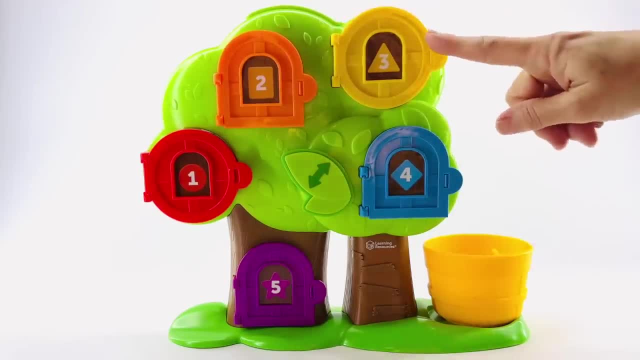 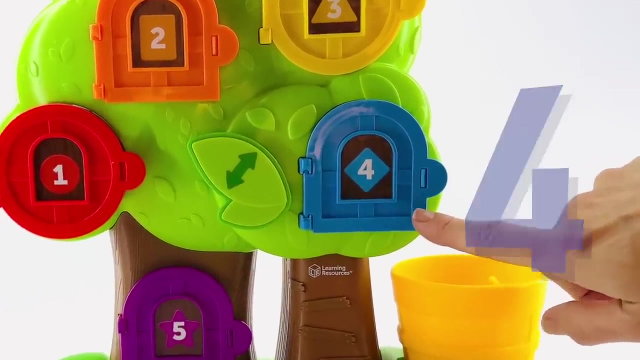 Do you know what number comes after the number three? Right, It's the number four. Do you see the number four here? Right, It's right here. That's the number four, And this door is blue. Blue in Spanish is azul. 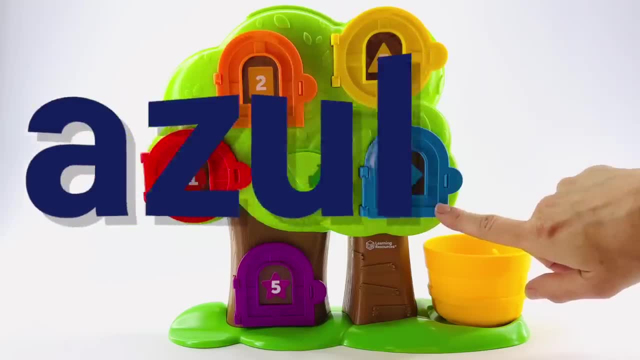 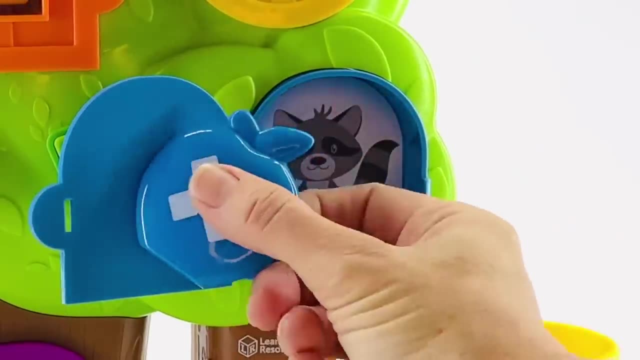 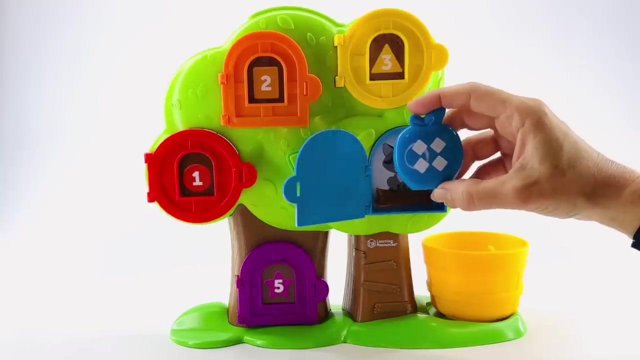 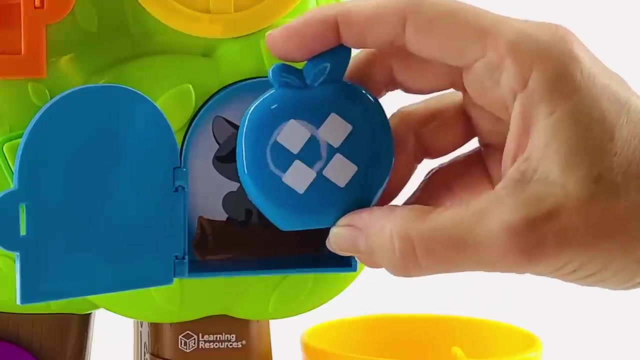 Let me hear you say it. please, Azul. Good job, Let's open it up and see what we have. Hey, It's another apple. This apple has diamonds on it. Four diamonds, Will you help me count? Great, let's do it together: One, two, three, four, Four diamonds. What do we do now? 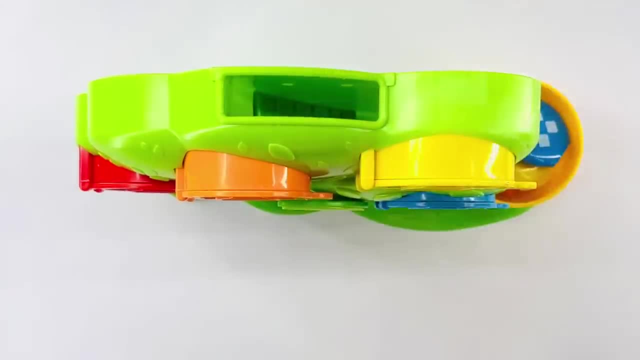 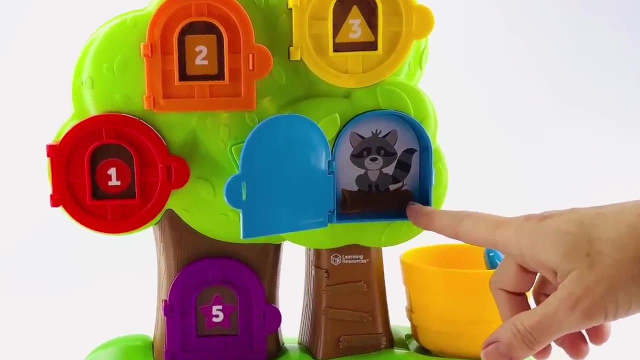 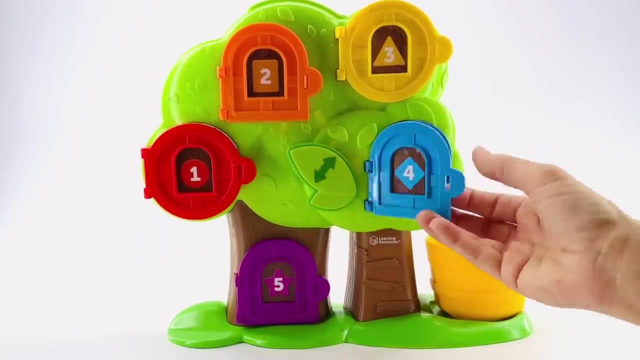 Right, We put it in the tree. Hey, what's that? That's a raccoon. A raccoon. The raccoon likes to make messes and it has black eyes that look like a mask. Let's close the door so he can go back to sleep. 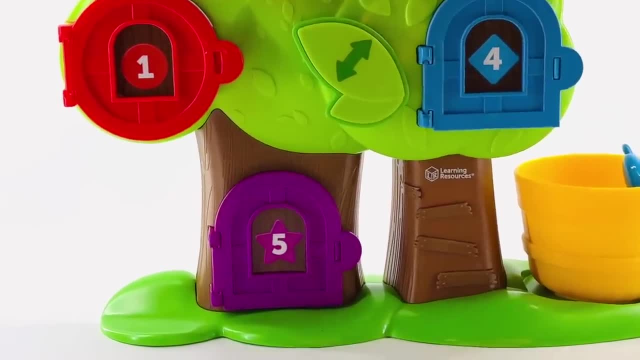 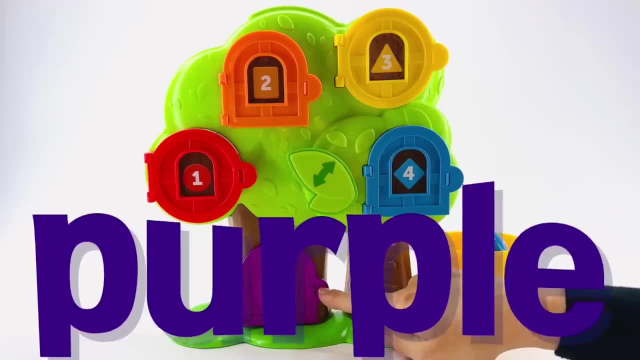 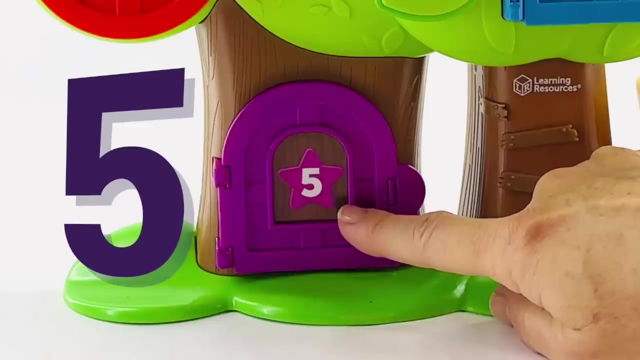 And our last number is the number five. Can you point to the number five? Right, it's right here. This door is purple, Purple, in Spanish is morado, And that's the number five. Okay, let's see what's inside. 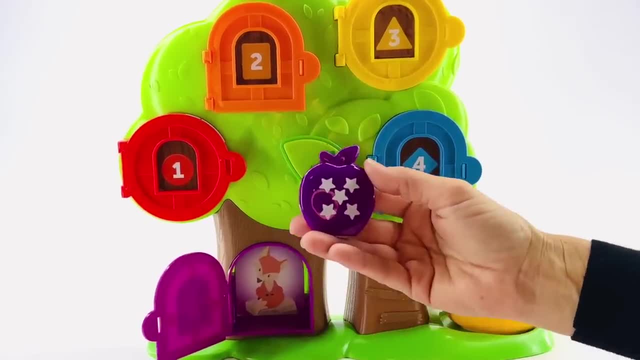 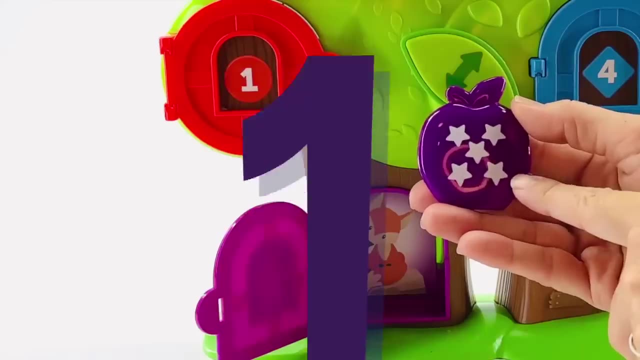 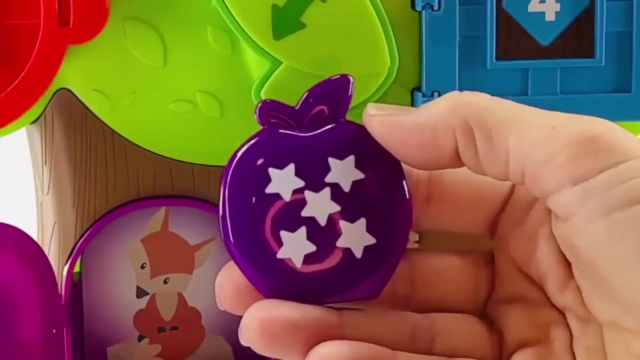 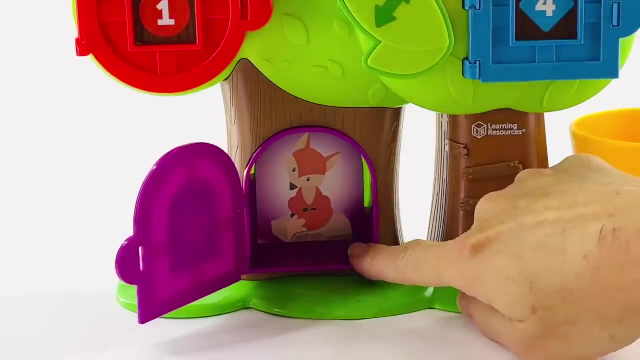 It's another apple. This apple is purple also and it has five stars. Let's do this one together: One, two, three, four, five, Five stars. Okay, let's put it back in the tree. That's a fox.